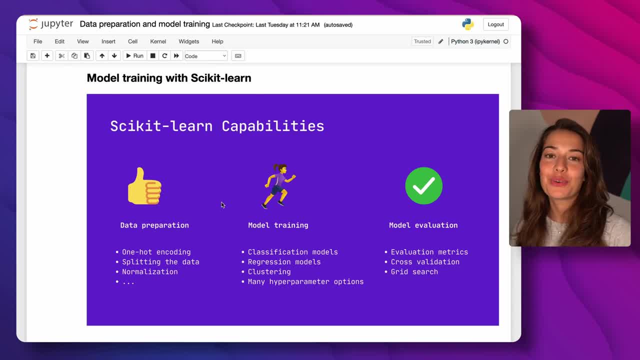 Hey and welcome again to the third lesson of our Python for AI development course. Today I'm going to show you how to train a machine learning model using the data that we prepared in the previous lesson using scikit-learn. again on Jupyter notebooks. Once again, if you want the data, you 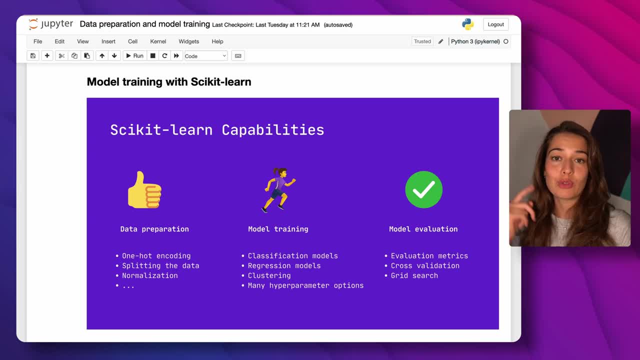 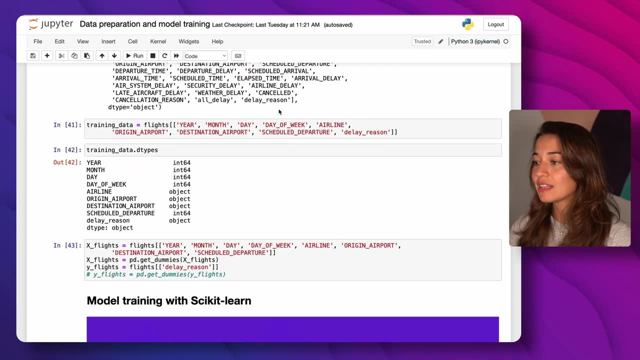 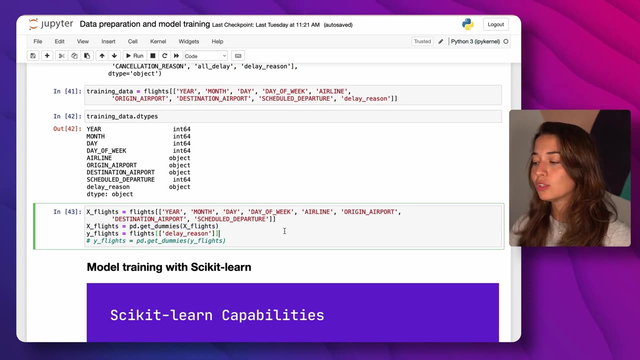 can go ahead and download it using the link in the description or I will also leave a link somewhere here on the video. If you remember, in the previous lesson what we did was lastly to divide our data set into x and y data sets, and we also created the one hot encoded version of this data set. 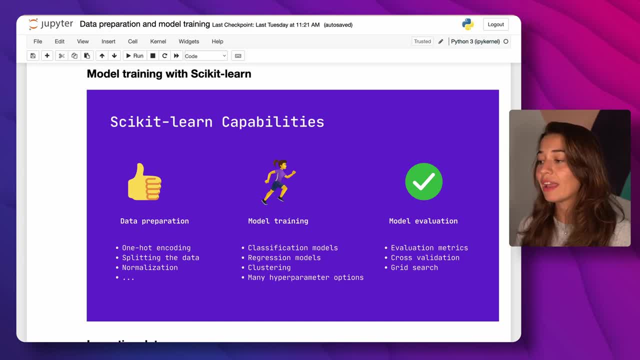 And today we're going to mainly use scikit-learn and, of course, Python. Scikit-learn is the machine learning library for Python. basically, There's a bunch of things that you can do with scikit-learn, but for a beginner level we can divide them into three main groups so you can prepare your data. 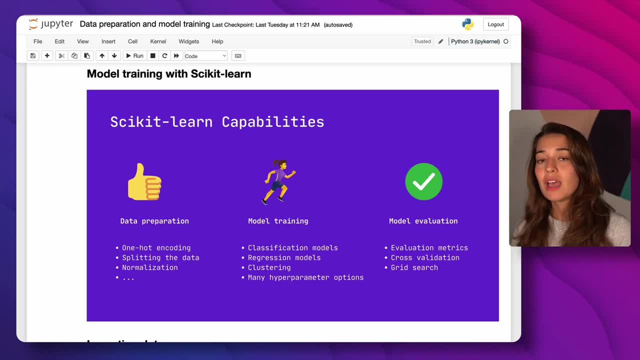 We already prepared our data to a certain extent with pandas, but here what the the. the main thing that we're going to do is we're going to divide our data into three main groups So you can prepare your data. We already prepared our data to a certain extent with pandas, but here what the the. 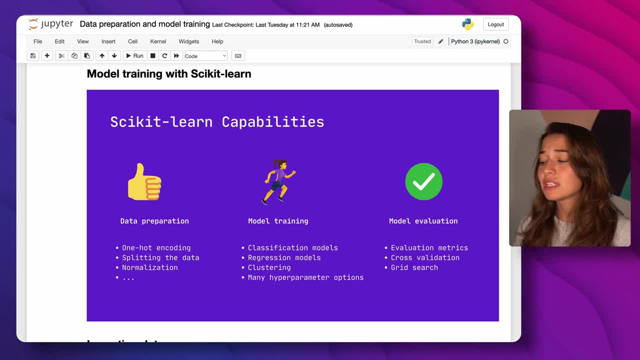 preparation I mean is you can also do one hot encoding with scikit-learn, or you can split the data into train test and validation sets, which we will see how to do. You can do normalization or maybe, if you're working with some other types of data like image or text data, you can also do. 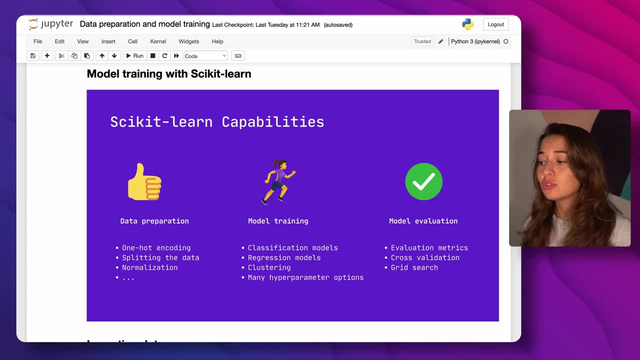 some other types of preparation for your data. Once your data is prepared, you can do model training. Scikit-learn by default has a lot of different types of models. You have clustering models, classification models, regression models and also for each of these models you have different hyperparameter options that you can set. 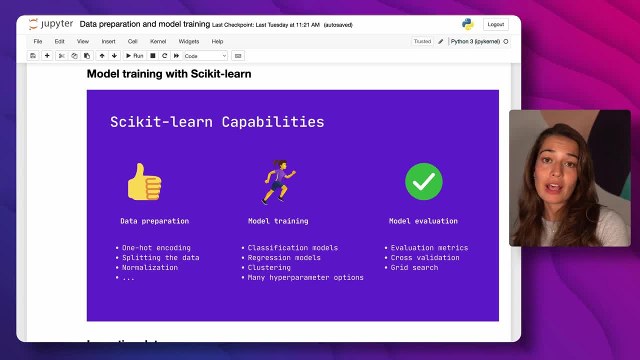 If you studied machine learning before, if you know about machine learning algorithms, you might know that each algorithm has its own settings. so that's what hyperparameters mean. If you want, of course, you can implement these machine learning algorithms, these traditional machine learning algorithms, from scratch. that wouldn't even be super hard, but of course it's. 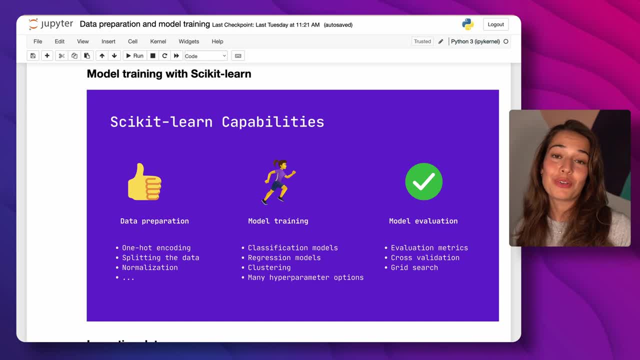 always easier to use something where you can create a model from scratch with just one code and then, using the hyperparameters, you can customize it and you can tune it to your specific problem. And lastly, once you train your model through scikit-learn, there is also a bunch of evaluation metrics that we can use. We will also see some of them today. 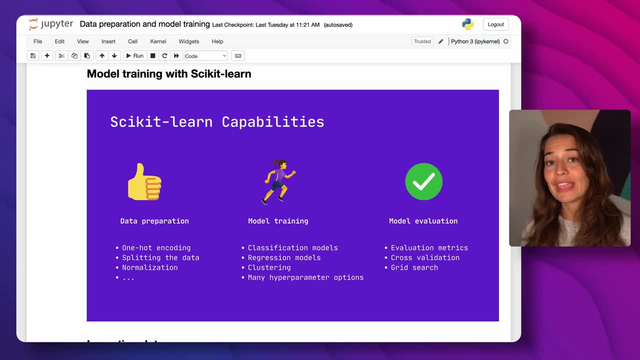 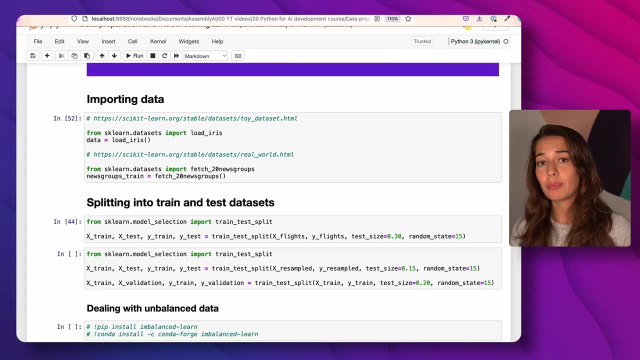 and using that you can try to tune your model and get to the best performance. One additional nice thing that we have in scikit-learn is actually data sets. So we already prepared our data set from Kaggle. so we got it from Kaggle and then we prepared it for. 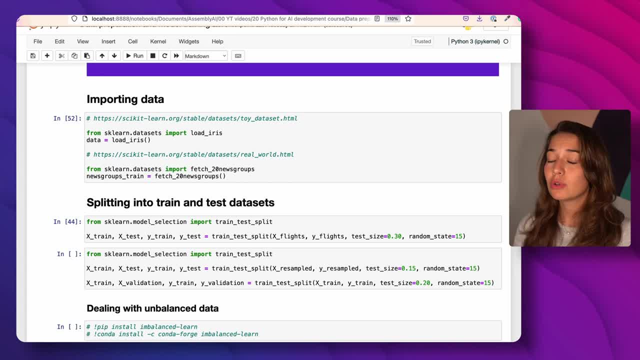 machine learning model training. But if you wanted to, you could use some data sets from scikit-learn library too. You have some toy data sets that are a little bit small. you also have a more real world data set that could be a little bit more unstructured, and they could also be. 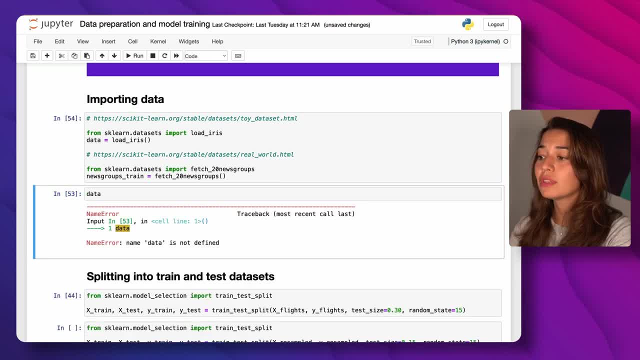 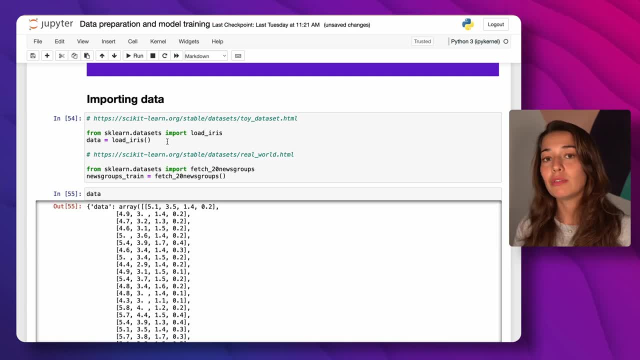 a bit bigger data set And the nice thing is they come with their own loading function. so instead of going and finding the data set and then downloading it to your system and like importing it again, you can just use the from sklearn data sets import load iris function and then using this load iris. 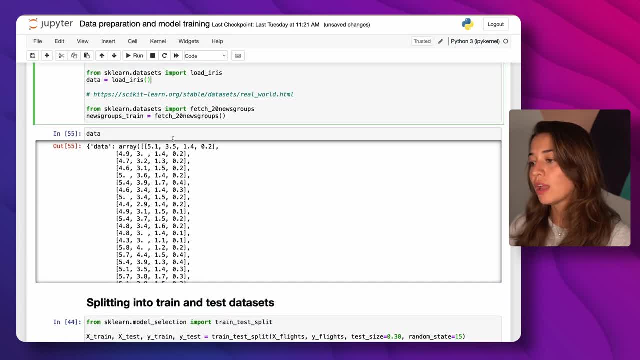 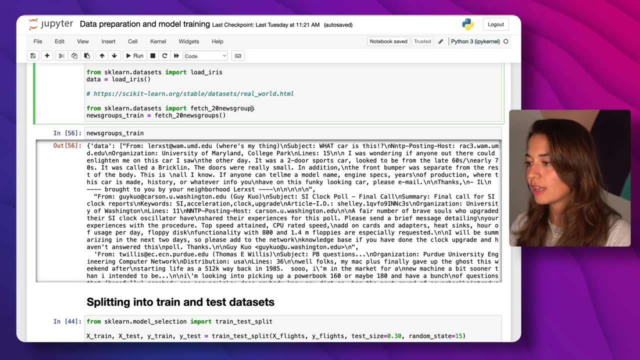 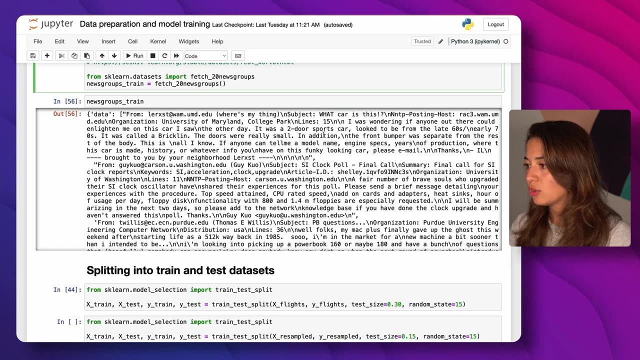 function, you can import your data set immediately to your notebook, And this is what the data set would look like. and then let's also see what the news groups train looks like, And this is a text-based data set. as you can see, we have information or text information from news. 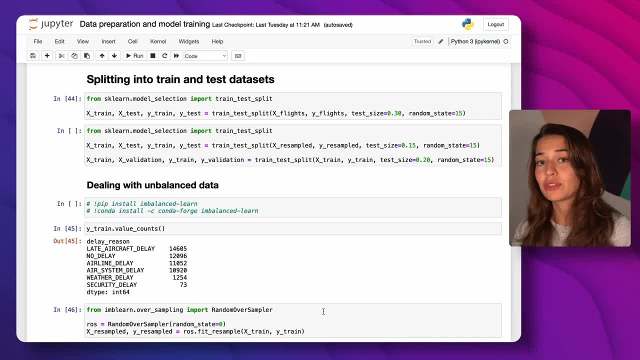 The next step that you have to cover before you train a machine learning algorithm is to split your data set. There are a couple of ways how you can do this. Sometimes you only divide your data set into train and test data sets, and sometimes you divide into train, test and validation data sets. 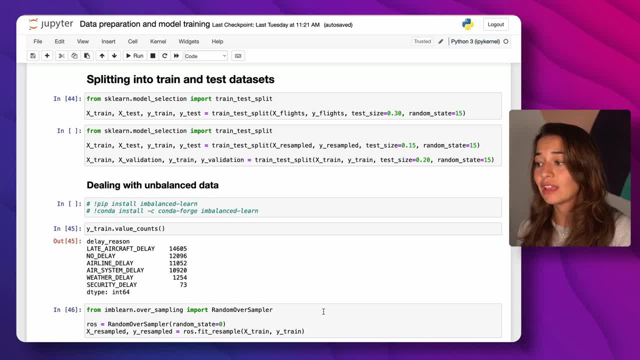 But you can do both using scikit-learn's train test split function. So if you only want to split your data set into training and testing data set, what you're going to do is use a train and test split data set, give your original x and y data sets and then tell the function how. 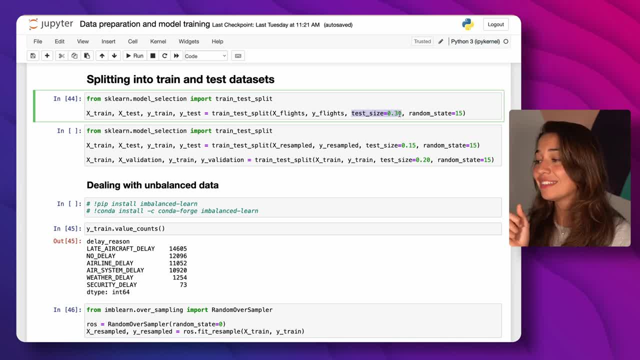 much out of one. what portion do you want the test size to be? So here I'm basically saying the 30 percent should be set aside for the testing data sets and you can also set a random state using this random state. next time you generate the data set again using the same. 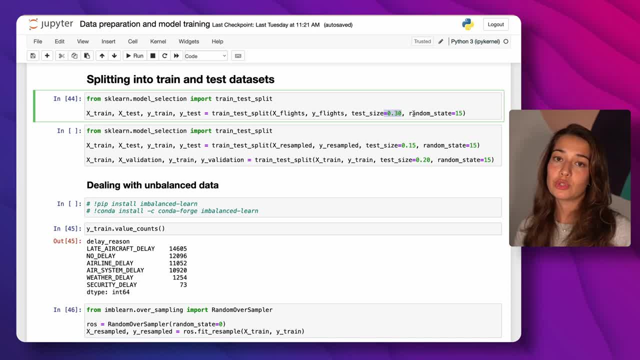 x flights and y flights, the same result will be returned to you. So if you want to keep the results same for your training and testing data sets- the same data points to be there- you can use that. If you want to instead create three separate data sets- so train, test and validation- 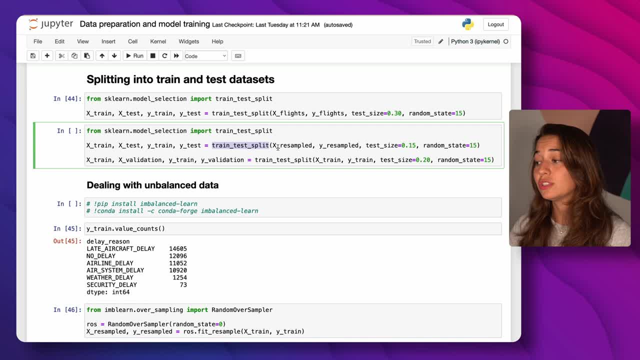 what you can do is to call the train test split function twice, So you can first create a train and test data sets, let's say by setting aside 15 for testing, and then what you can do is to call this function again on top of the train data set and then divide it into train and validation. 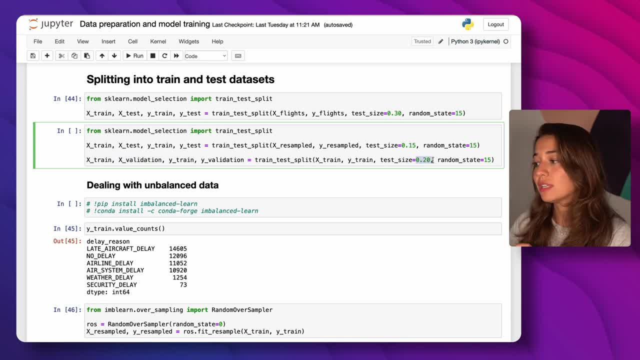 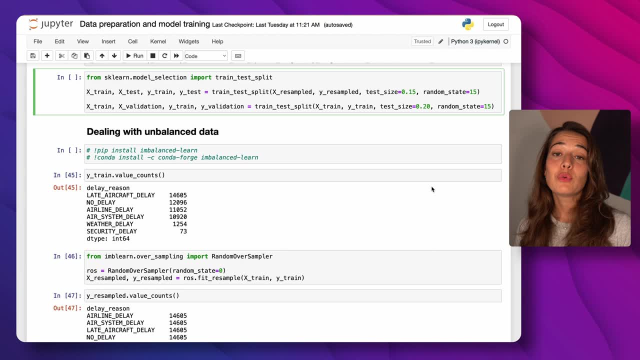 let's say by from the remaining 85 percent, you set aside 20 percent. So you can see that the training is now the same as the training and the test and validation data sets are the same size. And one last thing, before we jump into the model training is: if you have 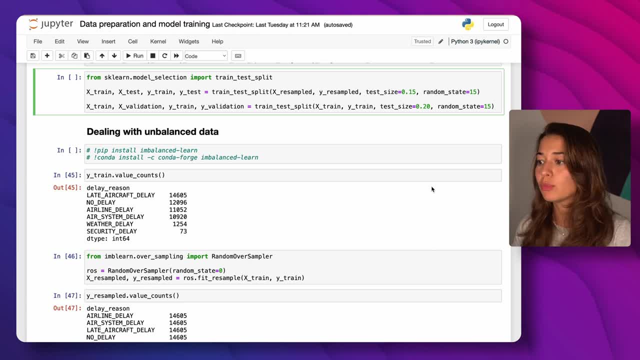 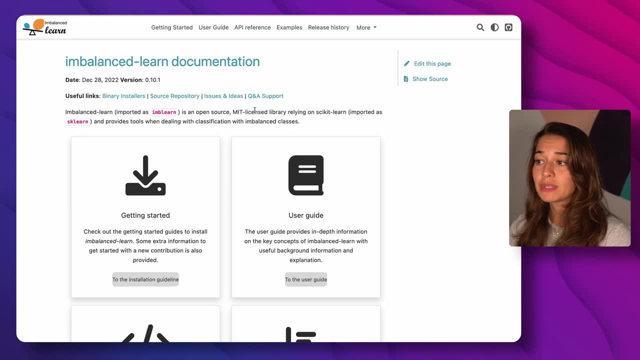 unbalanced data. you might want to deal with that before you start training your model. So there is a library called imbalance learn. you can see the documentation on their website too. it's called imbalance-learnorg. It's a very simple, easy to use library. what you do is basically. 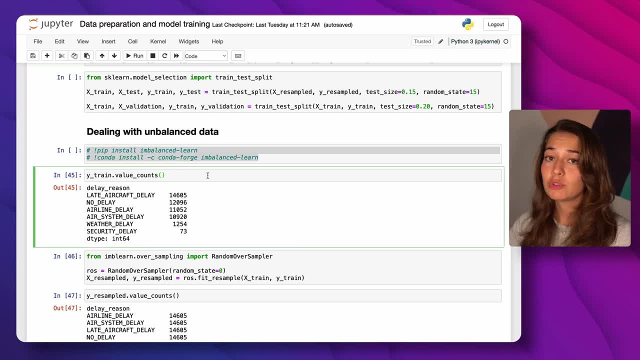 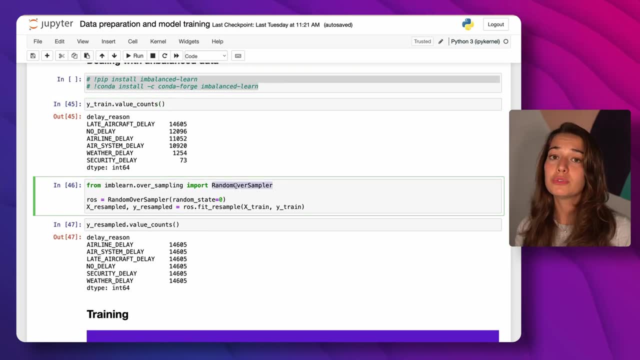 at first. you have to install it, of course, using pip or conda, Whichever one you're using, and you just need to call either a oversampler or undersampler. they have a couple of different options for how to sample your data set, but basically what happens? 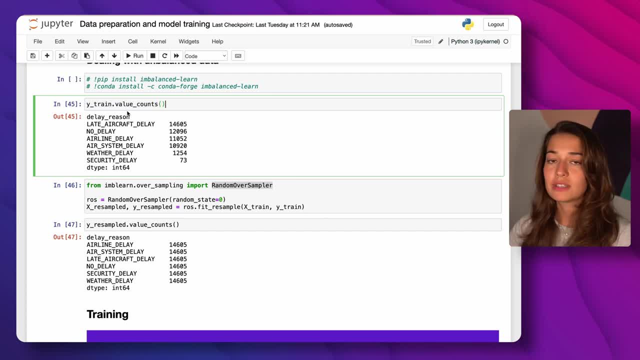 is. let's say, this is our train data set, this is the y train. so the target values. if we look closely we see that there these are one, two, three, four, five, six separate values that we might have or we have in our data set and we see that late aircraft delay happens. 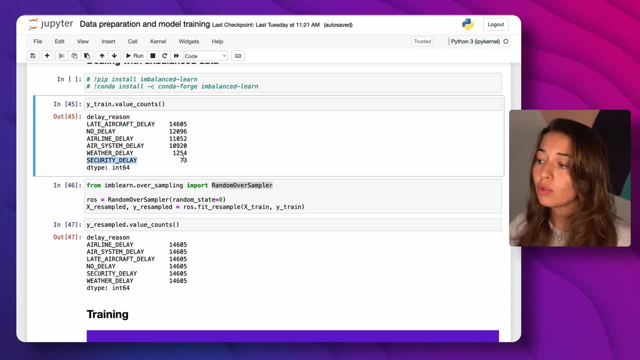 more than fourteen thousand times, whereas security delay only happens 73 times. So when you try to build a model on top of this, because of this imbalanced structure of the data set, you might not be able to get a train, a model that is really good. 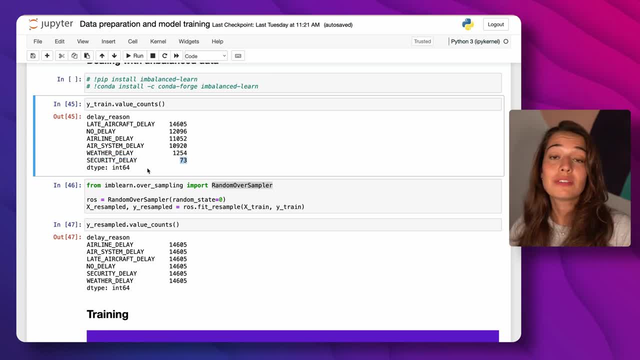 at um finding or classifying a instance as security delay. So, then, what you might want to do is to oversample it. so sample it more than once, each data point more than once, and feed it to your data set more than once, in hopes that it will actually create a more robust model that can 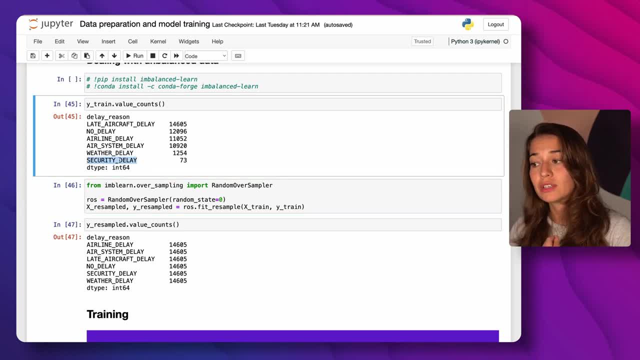 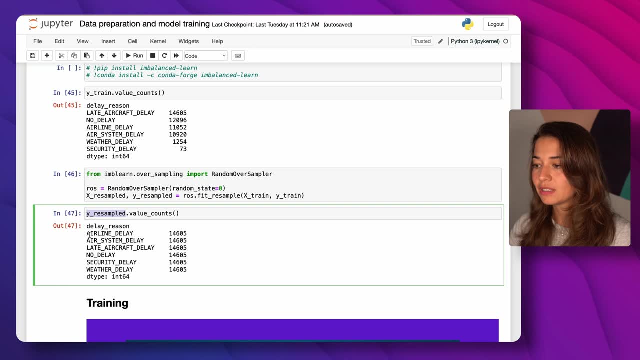 also, or that is also able to classify security delays correctly. So if you use oversampler, what you're going to get is, at the end: this is a resampled data set. you will. there are different strategies that you can use, but with the default strategy you sample all of these different classes so many times so that the amount equals to. 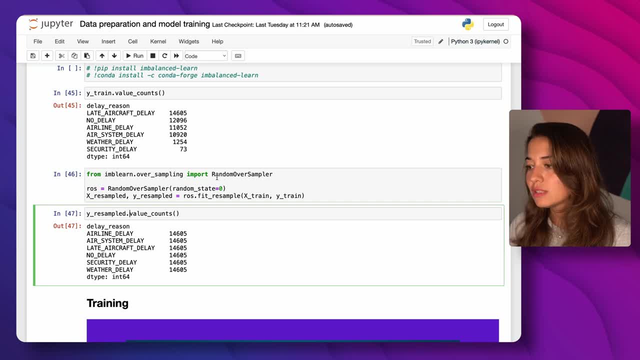 the majority groups amount. How you do it is. this time I used oversampling. from imbalanced learn. I import oversampling. as I said, there are a bunch of different ways to do oversampling, but the simplest one is to use random oversampler and again, if you want, you can give it a random state. 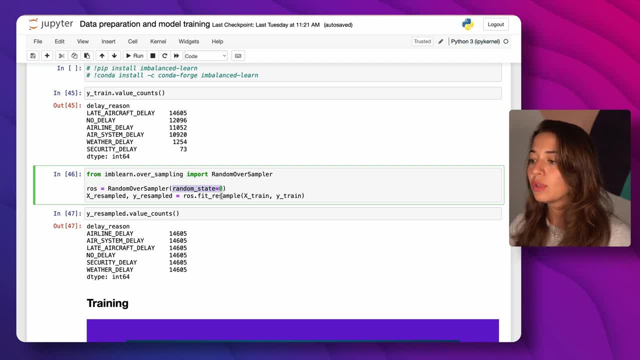 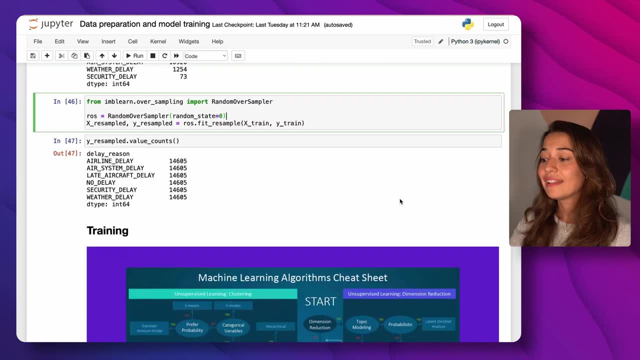 and all you have to do is basically to the fifth resample function. you need to pass the data sets or data frame that you're working with and then it will return to you the resampled data set. Next we have model training. this could actually be quite an overwhelming step, because it's kind of 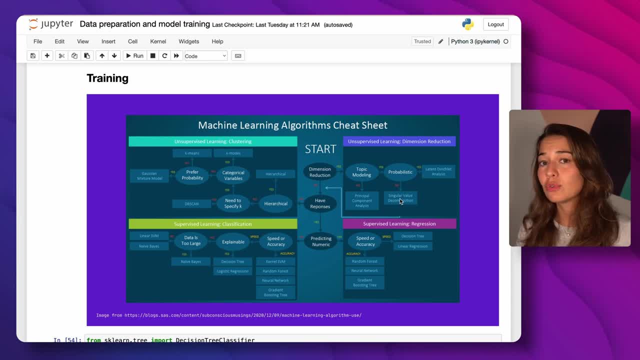 hard to know sometimes what kind of model you should go for. We have a lot of different models available in scikit-learn library but you know you can also implement some other models. One thing that I do, kind of my go-to approach, is once I decide on what my problem is going to be if 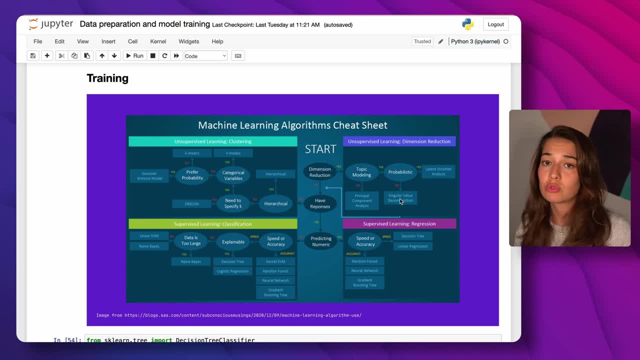 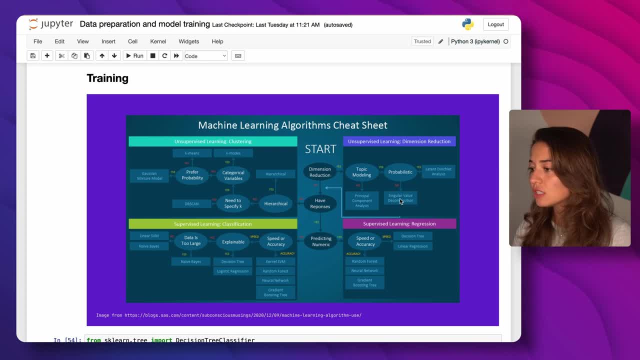 I going to prioritize speech? or am I going to prioritize speech or am I going to prioritize speed or accuracy? I go and take a look at this cheat sheet and then, by basically answering these questions, you can see which one you should try first. So, for example, if we do it right now, this is a diamond, this is not. 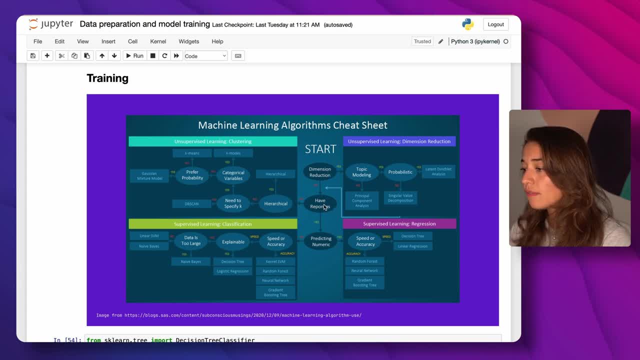 a dimensionality reduction problem, so it's a no. We do have responses, so it's a yes. We are predicting. we are not predicting numeric, because we're trying to predict the categories of whether the flight is going to be late and if it is going to be late, what is going to be the reason. 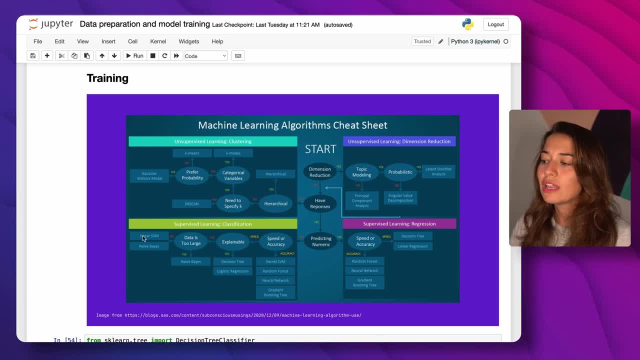 and once we're here, we can basically use any of these. but let's say I want to optimize for accuracy this time and once we're here, we can basically use any of these algorithms. but let's say I want to optimize for speed this time and I want it to be explainable. then I can try decision. 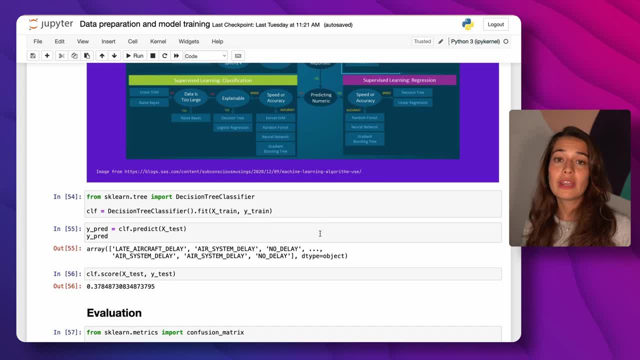 trees, for example, With scikit-learn training a model is quite simple, so all you have to do is from scikit-learn you need to go find your algorithm and normally in the documentation they do a really good job of explaining how you should import it. so I'll actually show you an example. let's say I want to use decision trees- regressor. 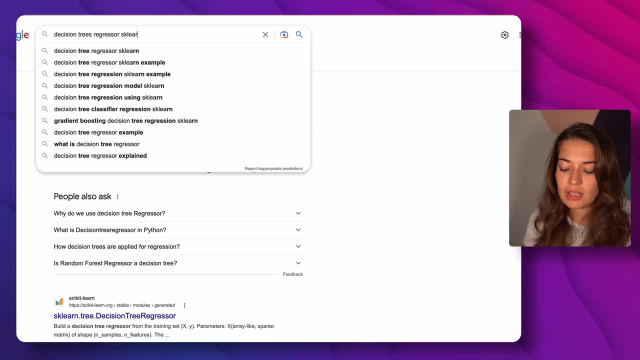 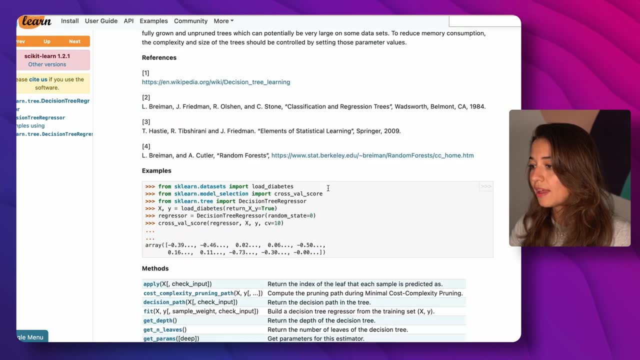 I can just search for decision trees, regressor, and maybe also add sklearn to it, and then I land at their documentation Inside the scikit-learn documentation. most of the time they have a little code example so you can see how you're going to import this. 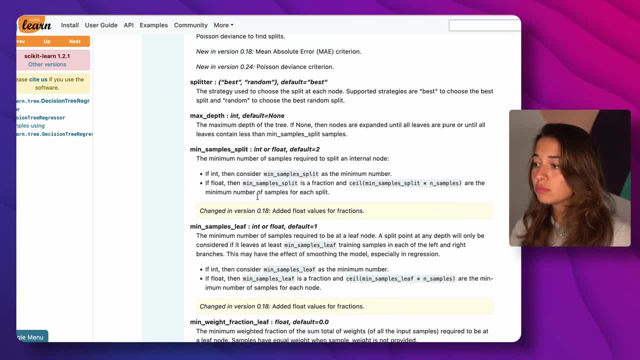 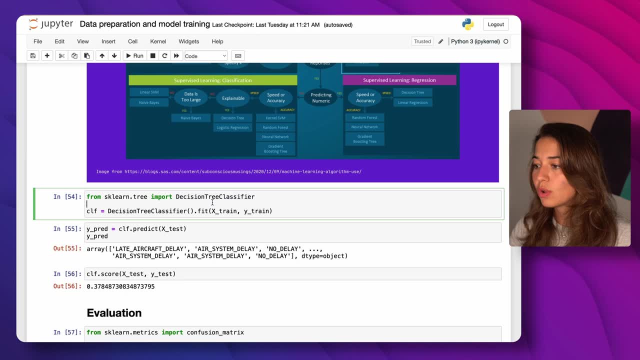 algorithm or model to your code. also, they have explanations of all different types of hyper parameters or settings that you can change. so then it's quite easy to just copy and paste that code here. all you have to do is to basically create a instance of this decision tree classifier. 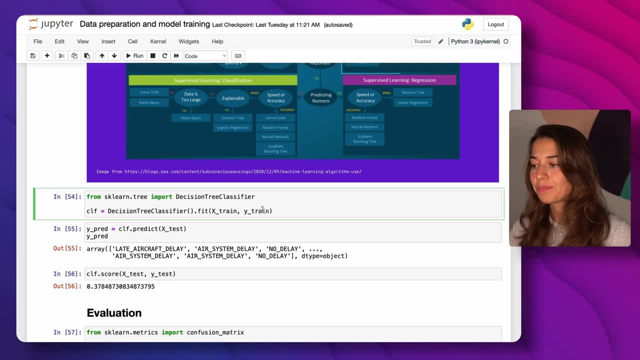 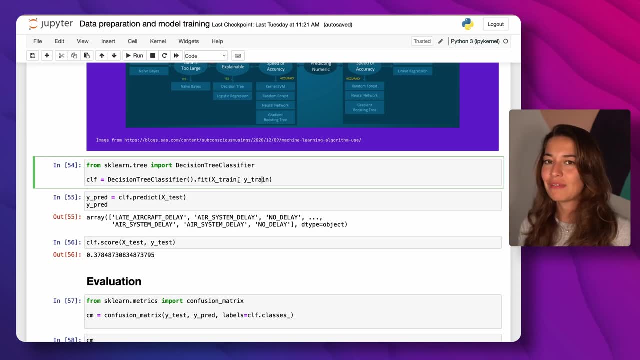 and then you call the fit function on it by passing the data to it. once you pass the data and once this model is trained- I trained all of this beforehand because sometimes they take a little bit too long, because you know we have a lot of data points- 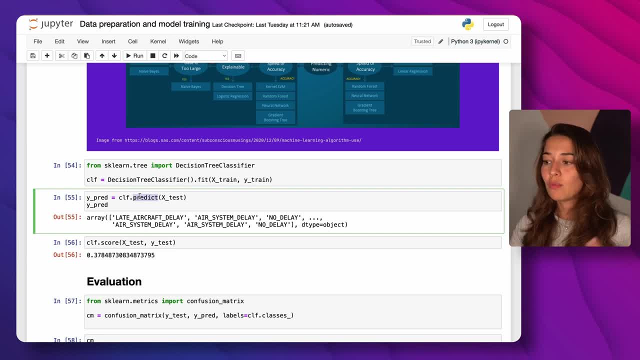 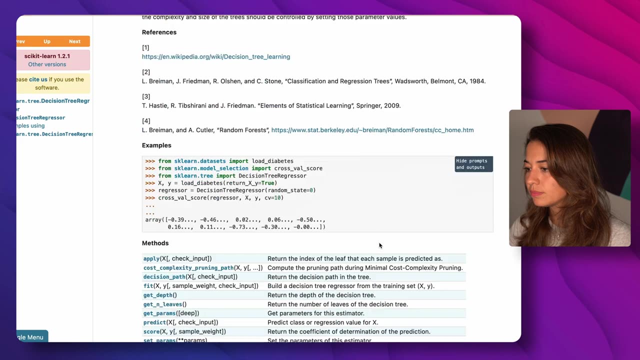 um, what you can do to get the results from it. so once this is trained, once this cell has run, the clf variable there contains our model. so to get predictions from this model you can simply use the predict function. this is also included in the documentation so you see what kind of functions. 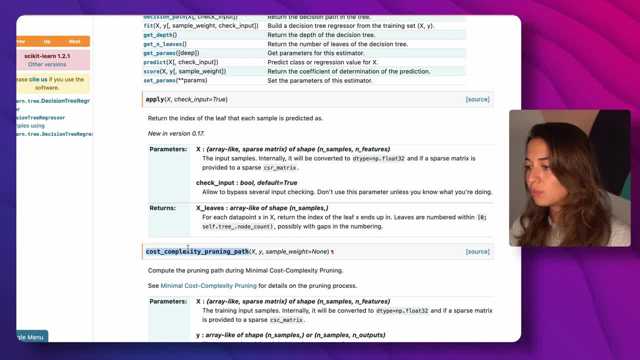 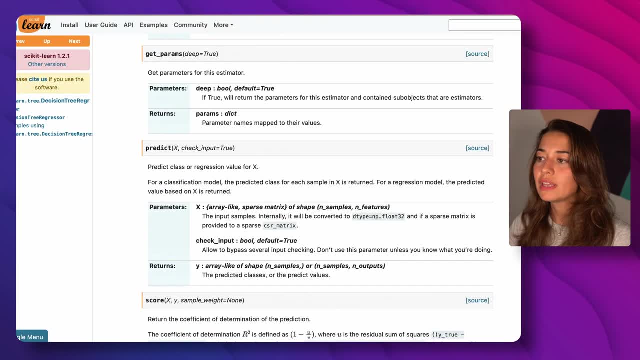 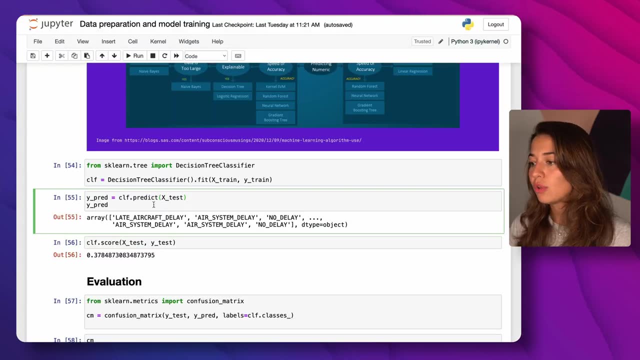 you can call on the model that is trained so apply cost complexity, pruning pad, decision path fit. you see all the predictions, predict score. all of these things, with their explanations, are in the documentation so you can see what are the possibilities of you can do with this model and when you do predict and when you 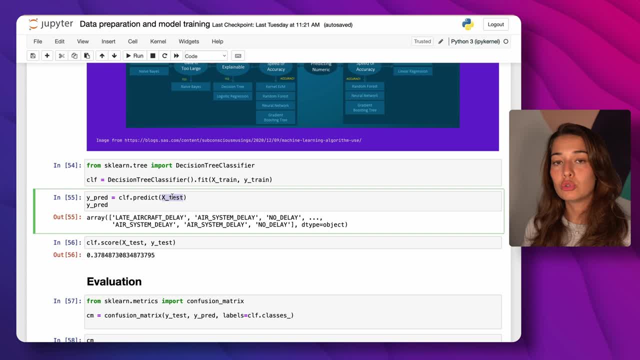 pass it. you can only pass it also just one instance, and then it will do predictions for that instance and you'll get the result. but if you pass it- a test data set, for example- it will do predictions on all of these instances in the test data set and then it will pass you. 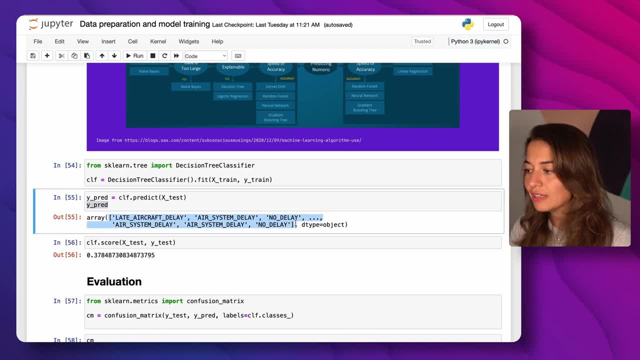 the predictions, and the predictions will basically look like a list. this list will be as long as your test data set and for each instance in the data set it will give you one answer. so it thinks the first example, first flight, is going to be late because of a aircraft delay. the third one is: 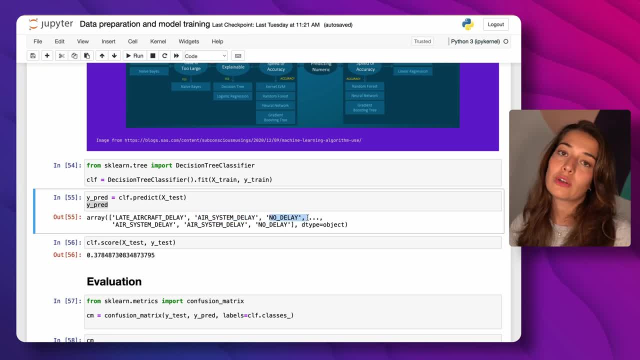 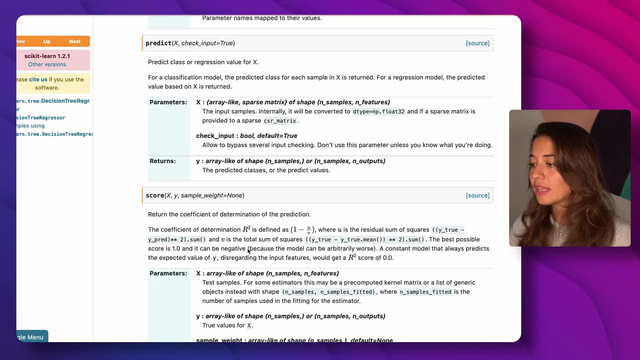 going to be late because of an air system delay and the third one is not going to be delayed. for example, and to see how well your machine learning algorithm that you just trained did, you can use a score, the one that we just seen here also, and here you can see the details. for example: okay, we're returning a score, but what is the score? 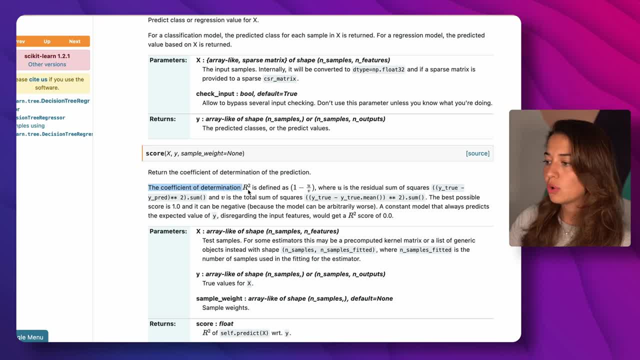 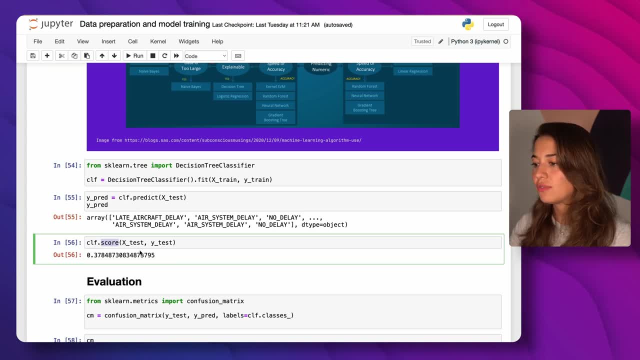 uh, and apparently here we're getting the coefficient of determination, so the r squared score when we are using the score function on top of our classification decision tree classifier. and to this decision tree classifier you just need to pass your x tests and y tests. so basically, what it does is it does the step automatically, it calculates your predictions. 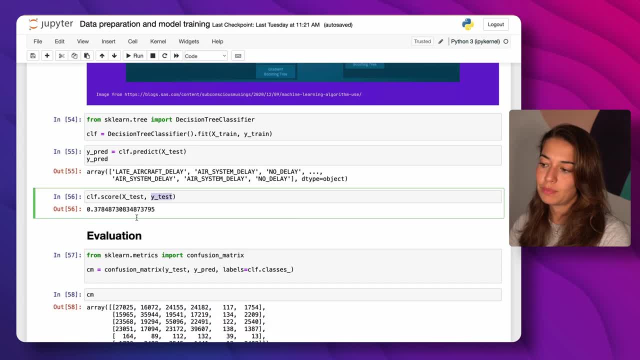 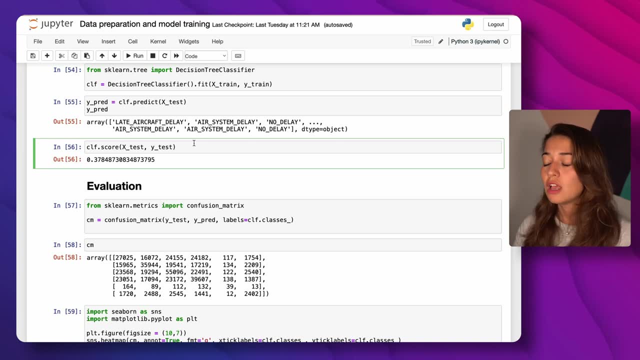 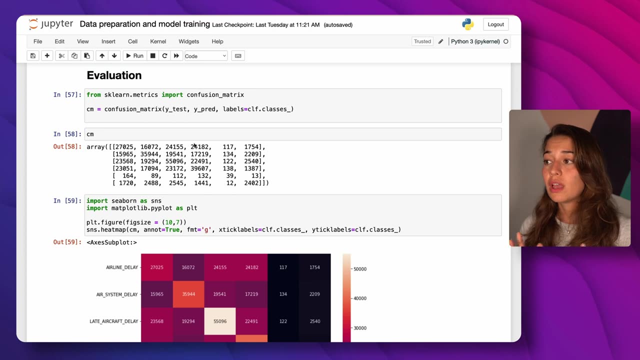 and it compares it to the actual values that that they have to be. But sometimes, of course, just one number, one score, might not be enough, especially in a case where we have multiple classes. So for that, what you might want to do is to include some other evaluation options. With scikit learn, there are actually a. 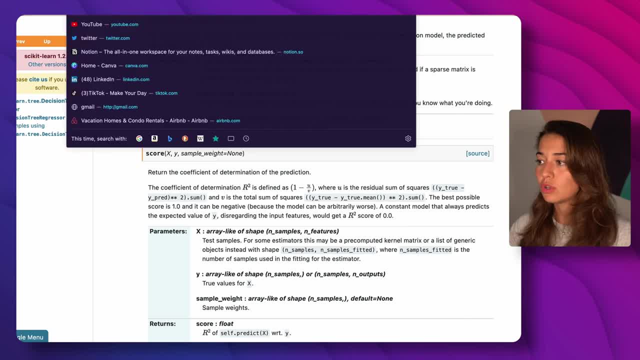 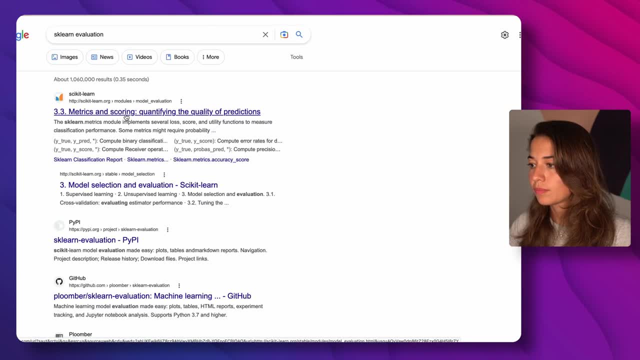 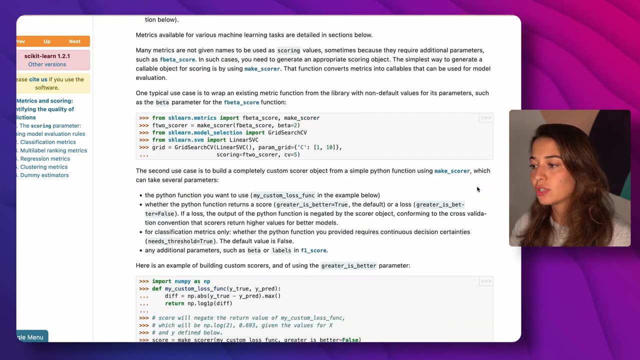 lot of different ways how you can evaluate your models, So we can also go take a look at the documentation there. So, metrics and scoring: if you go here, you will actually see a very big list of different types of metrics that you're going to use. Of course, it's always a good idea to 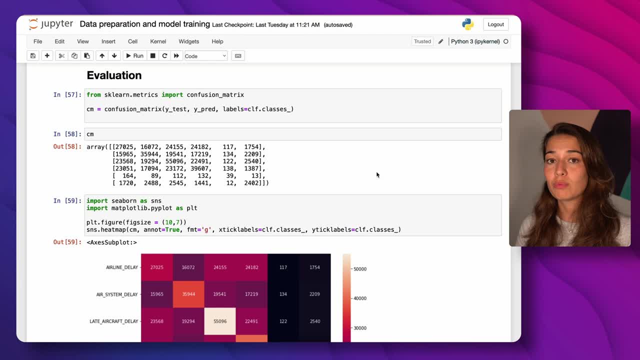 have in mind before you start your project, or once you decide what your problem is going to be, to kind of what metric you're going to be optimizing for. But even if you have no idea, you can kind of go to scikit, learn, or maybe just to learn something. 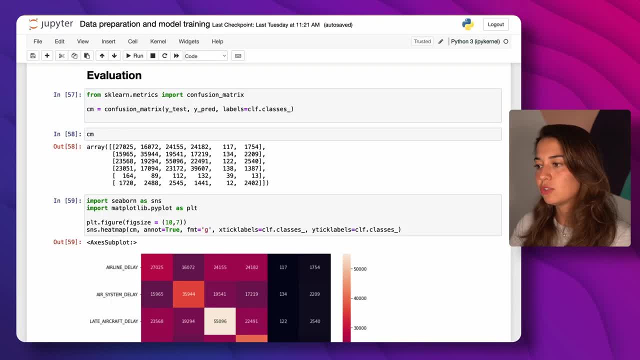 You can go to scikit learn documentation and to understand what metrics you can use. So in this case, in this multi class case, one thing that I like to use is a confusion matrix. Again, scikit learn provides a confusion matrix algorithm to calculate the confusion matrix values And what. 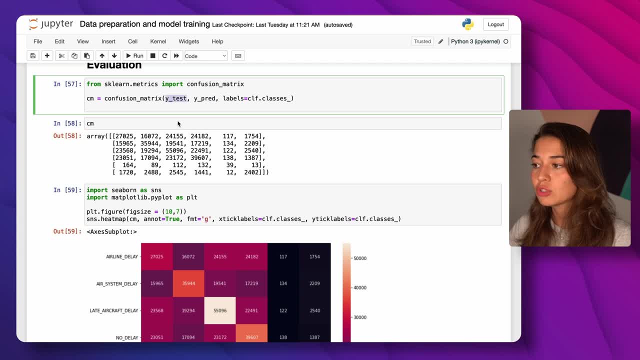 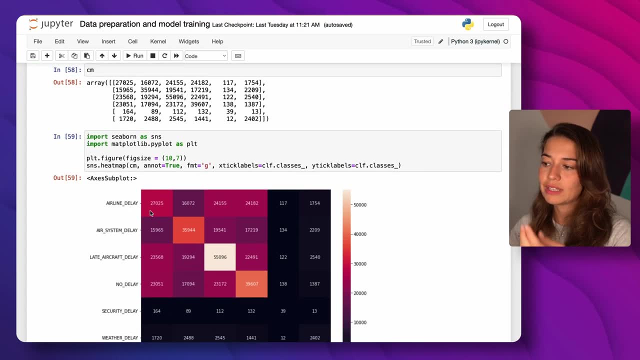 you do is you pass it the predictions that you calculated and you also pass it the test. So the actual values And, if you like, you can also pass it the labels of your classes. So basically, airline delay- aerosol system delay. 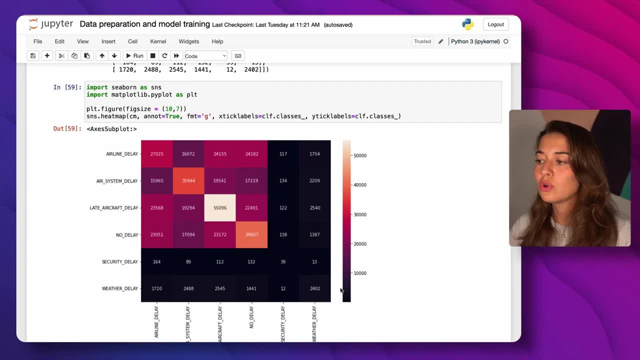 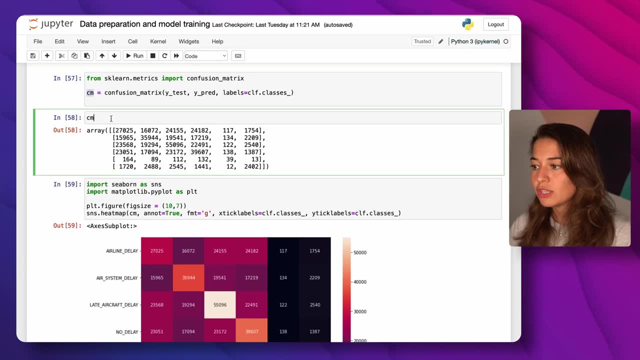 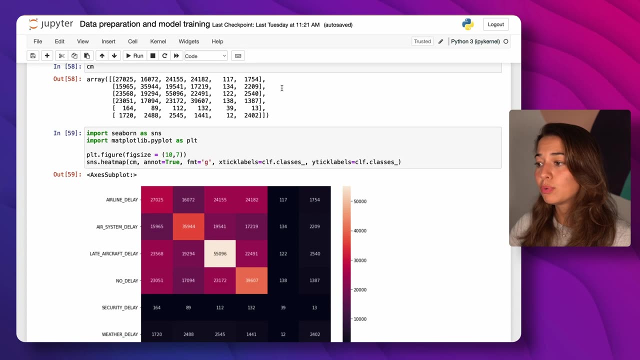 no delay, security delay, etc. So that when you produce your graphic it's going to look nice and clean instead of just having numbers there. Once you calculate a confusion matrix, it's actually just going to look like these numbers. So that might not make a lot of sense to you. That's why I like to use other plotting. 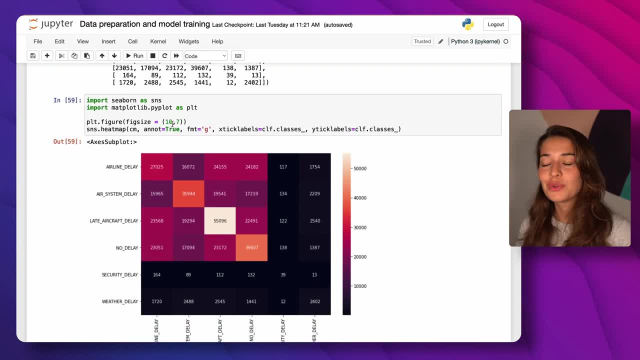 libraries, for example Seaborn, which creates some nice and colorful graphics for us. And here what I do is from matplotlib. I am creating a canvas using matplotlib, matplotlib and Pi plot, and on top of that I am creating a heat map from Seaborn. And to this heat map I'm passing. 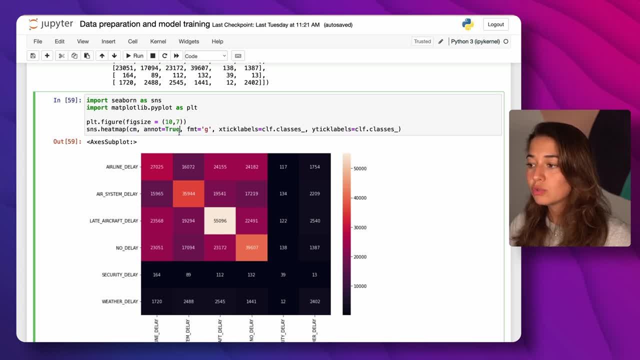 my confusion matrix. I'm calling my annotation to be true, so I want there there to be specific numbers and not just coloring in my heat map. This determines whether to show numbers fully or in a scientific annotation way, and for x axis and the y axis I am passing it the labels. So let's take a look at that. 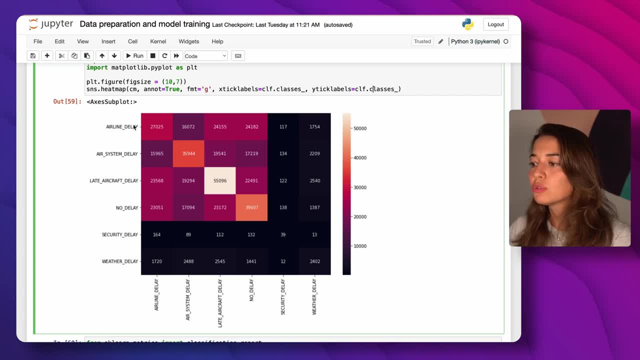 a look at this if you've never seen a confusion matrix before. it basically shows me, for every instance that was airline delay, how many of them were classified by the model as airline delay, so correctly. air system delay, late aircraft delay, no delay, etc. etc. so basically every value in this. 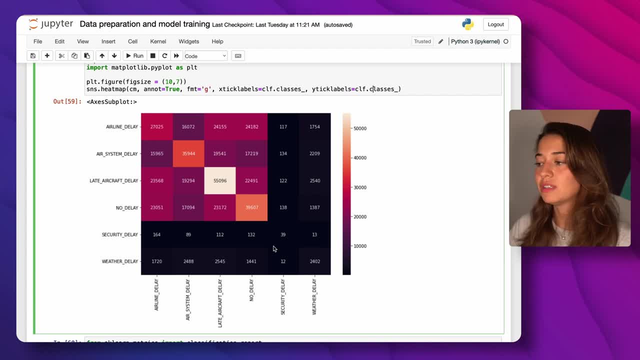 diagonal line shows us the correctly classified information. so how many of this information was correctly classified? so it looks like for the first four we actually got a good amount. and also the colors are determined, as you can see here, as how high it is. so ideally we would want 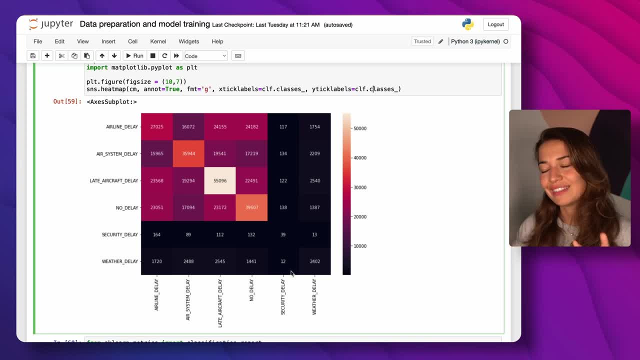 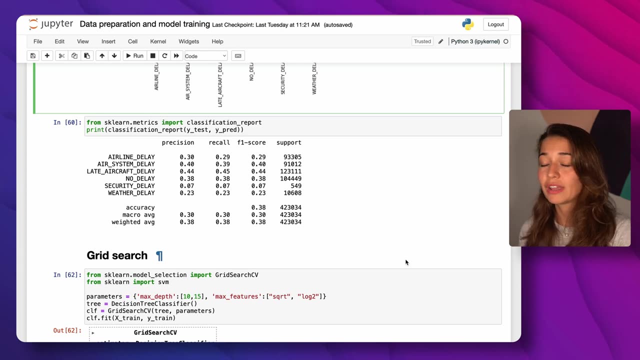 the diagonal line to be quite bright and the less the rest of the heat map to be quite dark, and that will show us how well our algorithm is doing, how well our model is doing. if you want, on top of that you can also create another report, which is called a classification report, directly. 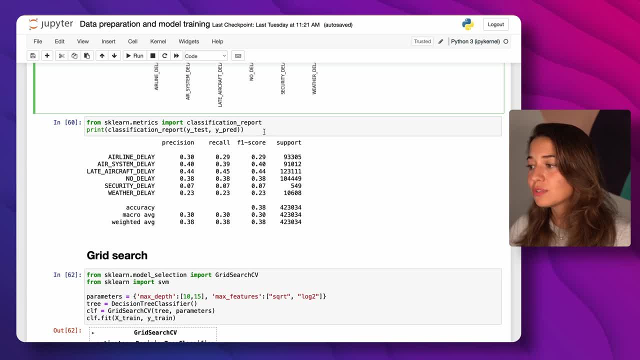 from scikit-learns- again super useful, and what it does for you is to create for each of your classes, and also, on top of that, for all of them together, what is the precision, what is the recall and what is the f1 score. and this is really useful, especially in an unbalanced case where we have 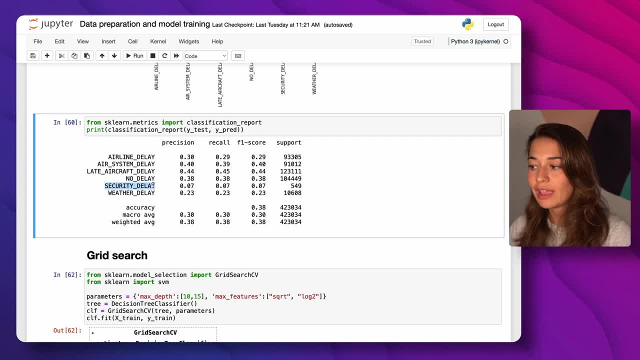 for example, not that many cases of security delay. you can see specifically how well you did for this class, because if you just get one number, if you just get accuracy, for example, you will get accuracy for the whole data set and what's going to happen is, if you have a majority class, you're going to 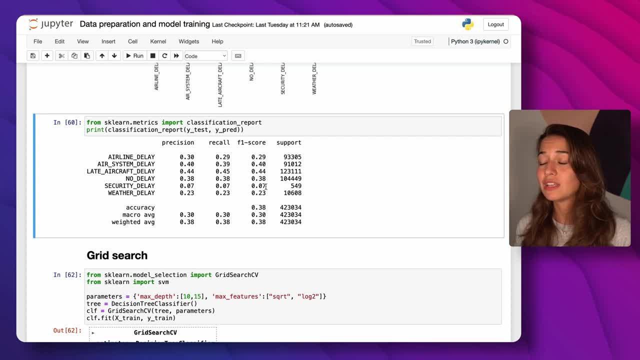 get 90 percent of your data set. and if you get 90 percent accuracy you might think, hey, i'm doing really well. but maybe the rest of the 10 percent is because you were not able to classify your minority class correctly at all. so that would actually give you, that would mean you have a 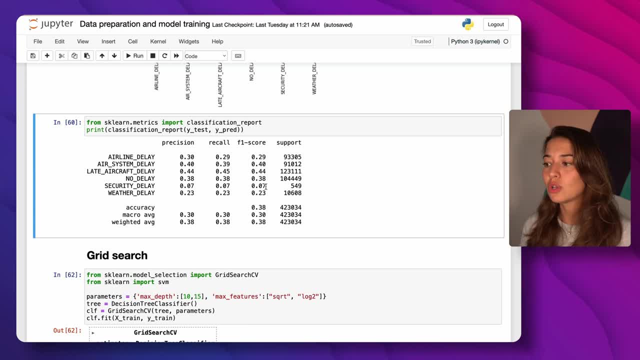 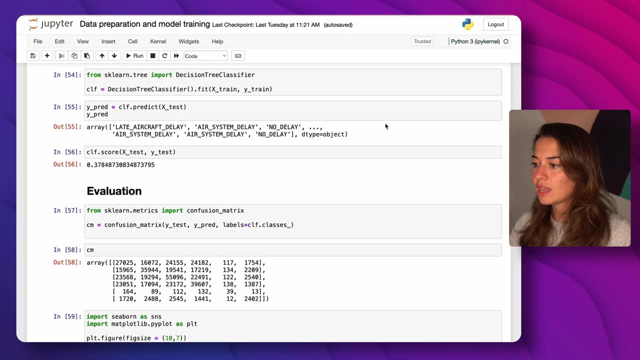 really bad model, but on paper it will look like it is a good model. so, especially for multi-class cases and when you have unbalanced data, make sure to look into a bit more details of your precision, overall precision or recall or accuracy. so so far what we've seen is basically to train the model. 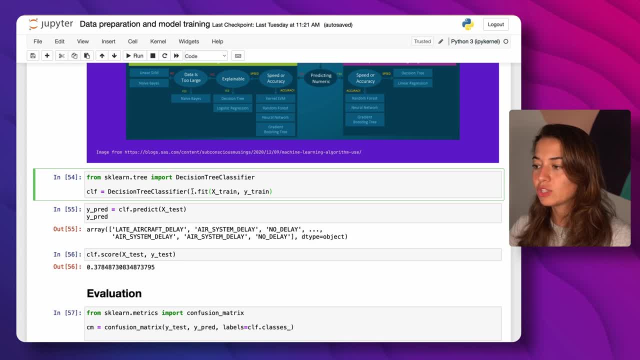 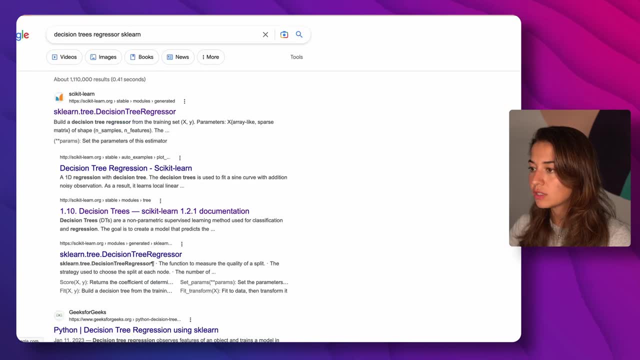 in one way you get the model right now. we are not changing anything about the model. we are using the default values for everything, as i said. just to kind of remind you, let's go back to the decision tree regressor, for example. it has many different options, many different hyper parameters that you 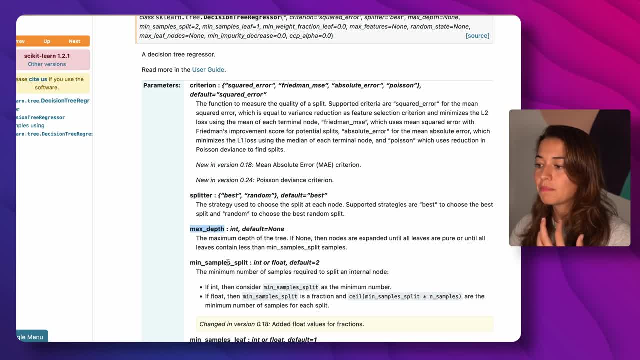 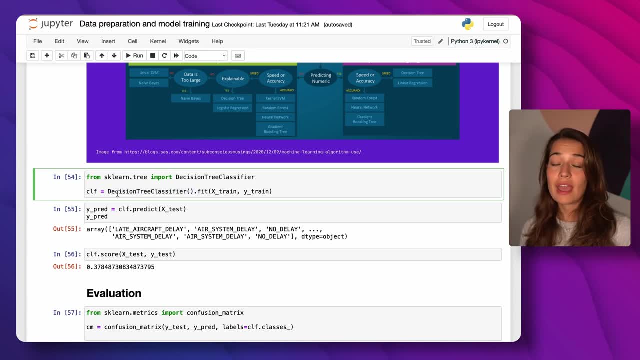 can set. so the criterion splitter, max steps, min sample split. but we did not change anything, so we are only using a default values here. but to build a accurate model you need to change these values, you need to play with them, maybe tune them a little bit and then see what gives you a better result. there are a 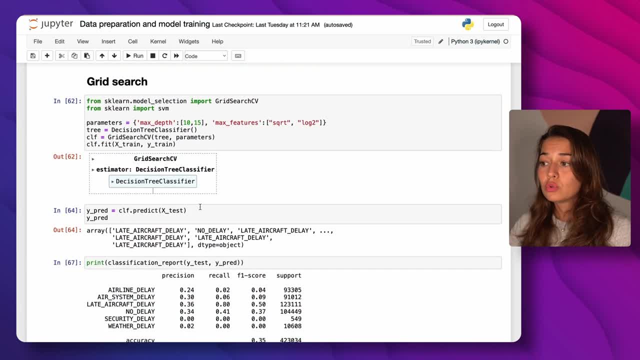 bunch of ways how you can do that. one of them is to do searches around your possibility space. so let's say, if you have four different hyper parameters and they all have two values, you would have 16 combinations of how you can make a new model. so you would have 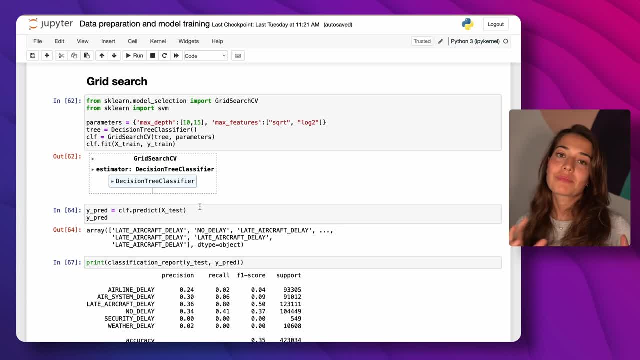 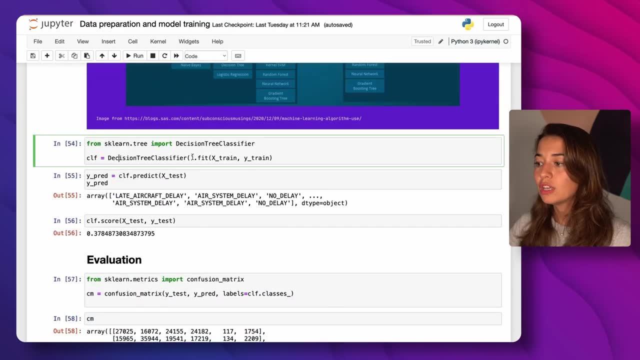 16 combinations of how you can make a new model. so you would have 16 combinations of how you can make a new model. so you would have 16 different options for making this model. and it is sometimes hard to go search through all of the space, because then you would have to make a new line for each of. 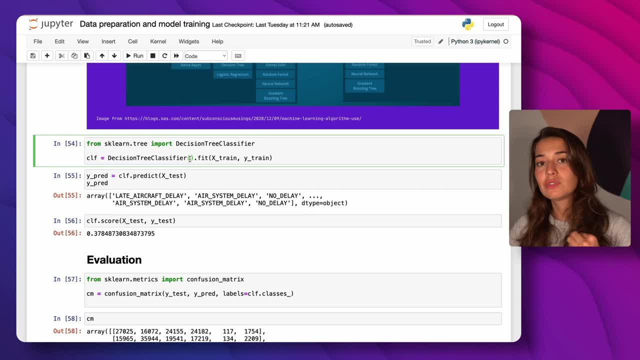 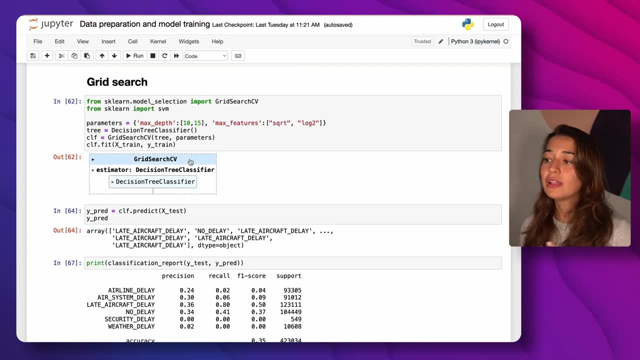 these models, change the settings and then save the results, save the predictions and then compare it to each other. instead, you can use the grid search from scikit-learn. there are also some other searching algorithms that you can use, but this is the simplest one, just to kind of get you started. 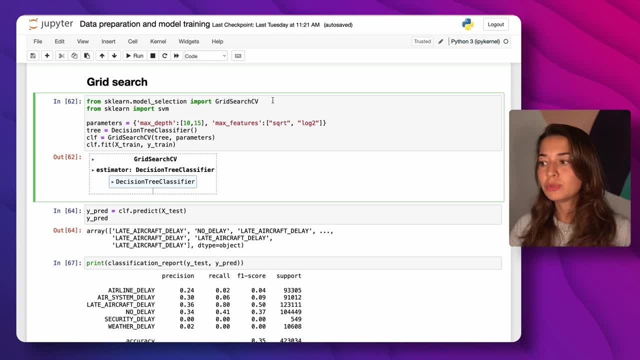 and what it does is to. you can use the grid search from scikit-learn. there are also some other searching algorithms that you can use, but this is the simplest one just to kind of get you started. all of these options that you give it for the hyper parameters. 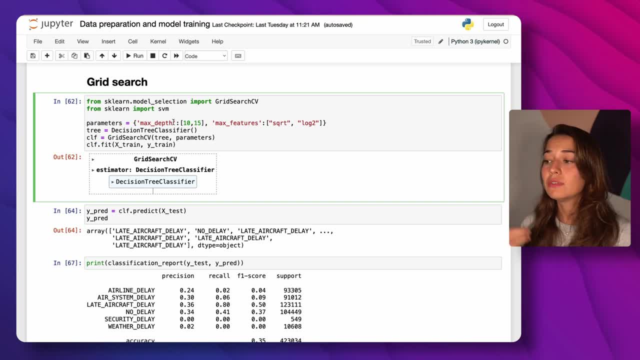 it creates a new model, it trains it with the data that you're giving it. it then creates the results from it, creates the predictions from it and all of these models. it compares with each other and then gives you back the best model, the best performing model. how you're going to set it up is, again, you. 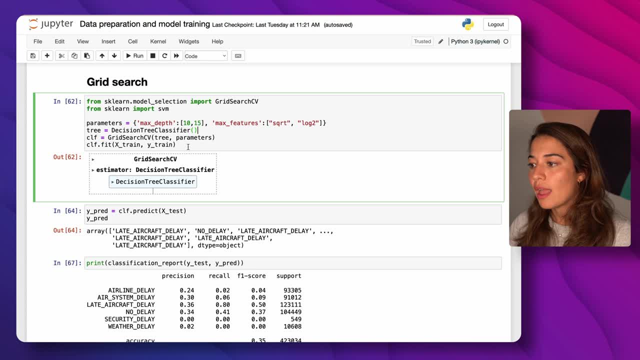 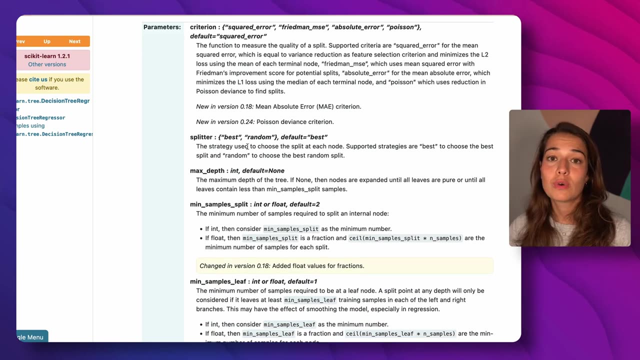 create your an instance of your model and you pass this instance of your model to the grid search cv and on top of the model, you also pass it some parameters. so, as i said, there are already a lot of different options of what you can set, so you can choose which ones you want to try for. 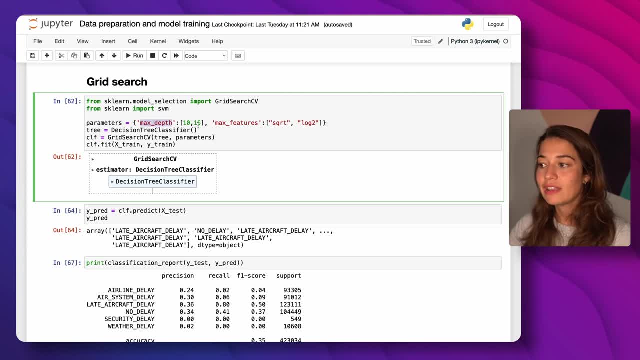 and then you can say: i want to try for max depth- 10 and 15- and for max features. so what should be the way to choose how many features are going to be selected for the next split in our decision tree? i want to try two different ways of determining that number and in total there will be four models. 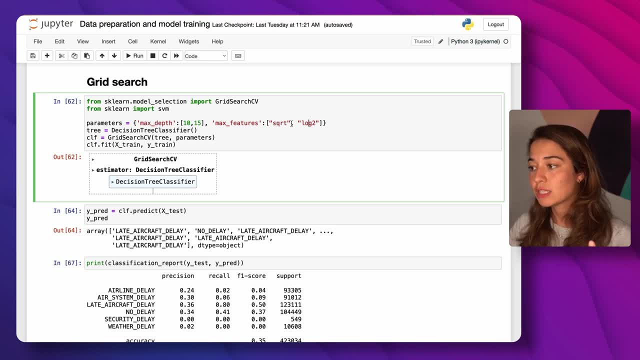 that will be comparing you with each other on the train. so one with where the max depth is 10 and max features is square root, one with max depth is 15 and the max features a square root, one where max features a max depth is a 10 and max features is log 2, and another one where max depth is 15 and 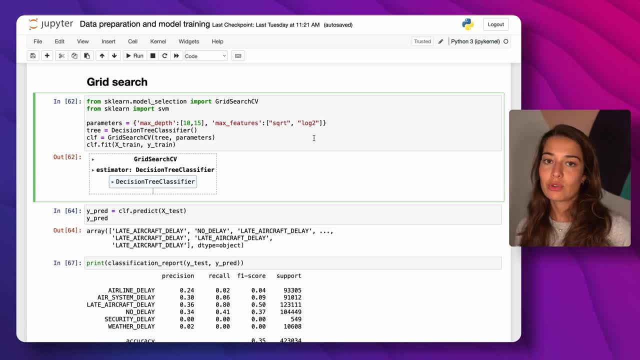 max features is log 2.. so in total, four models will be created like this, and then they're going to be compared to each other. and once i say fit on the train, and why? train data sets. using these data sets, it's going to compare these models to each other and 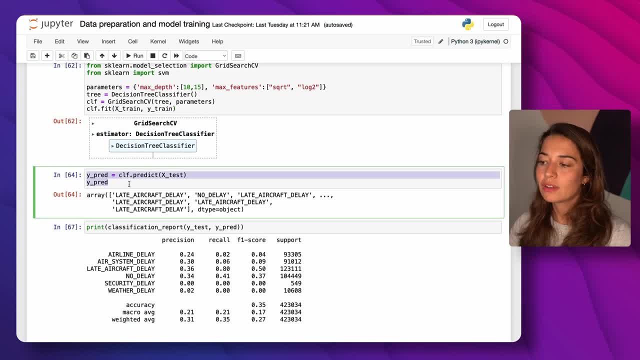 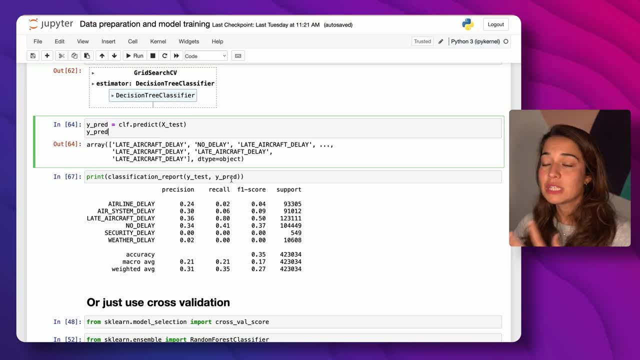 then return to me the best model And again, I can create the predictions from this model, like we did before, and see a classification report and maybe compare it to the base model that we just trained without changing any of the settings and see if there is a improvement. If not, you can. 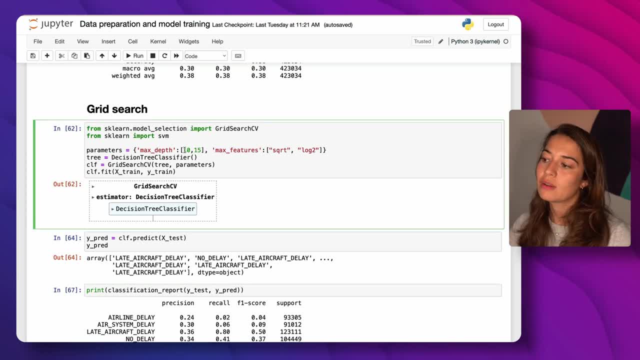 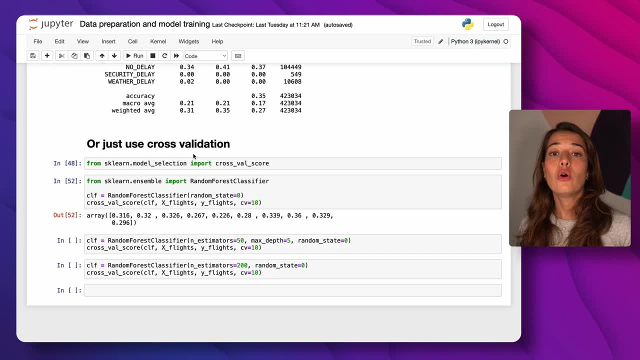 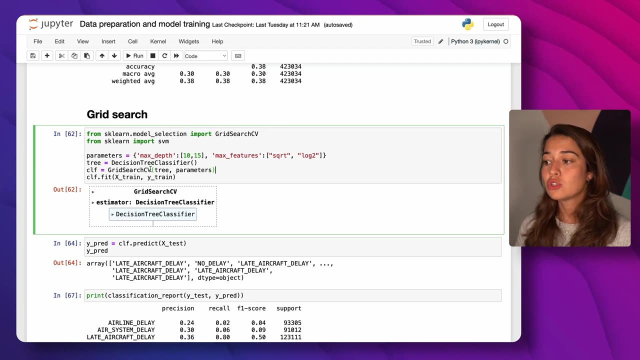 change where you're searching. you can add a new parameter here, you can include or increase the number of different combinations that you're trying out, or you can just cross-validation yourself. One thing I forgot to mention with GridSearch is that it includes cross-validation. 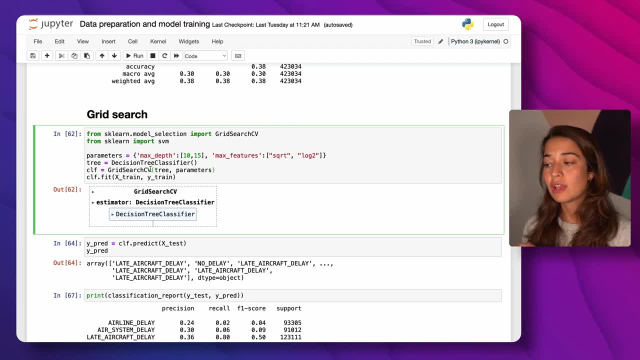 So, as it trains these models with these combination of parameters, it doesn't only train them once You pass it- the x-train and y-train- and then it divides it into subgroups and then trains a bunch of different models with the same parameters. 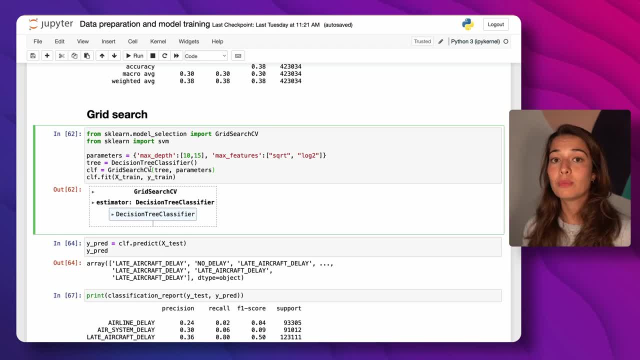 So each model is different and they all have the same parameters. So if you want to improve the And then the resulting, the actual performance, metric performance value of this model is going to be the combination of all these little models, So it is already done in grid search. but if you 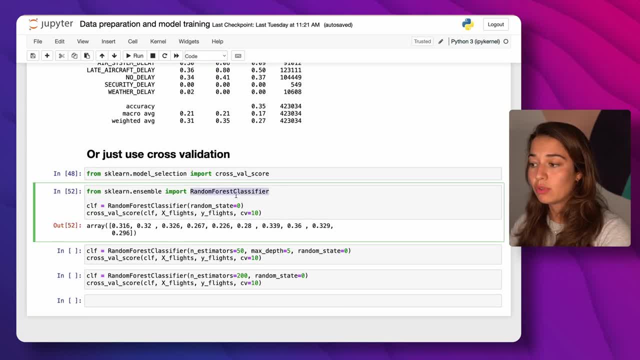 want to do it yourself. you can again get a model, for example random forest classifier, and then you can set the random state or not. You can. if you want, you can set some of the hyper parameters, for example number of estimators, max depth, or you can leave it as default again and then you can. 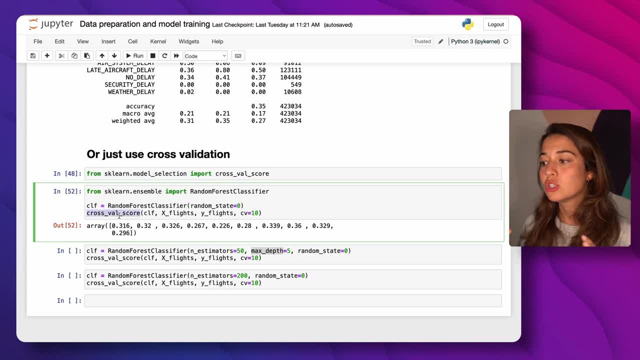 you can ask for the cross-validation score. So what it does is to the cross-validation score function. you pass how many times you want there to be cross-validation, so it's called k-fold cross-validation. If you pass it 10, it will be 10-fold cross-validation and the model that you 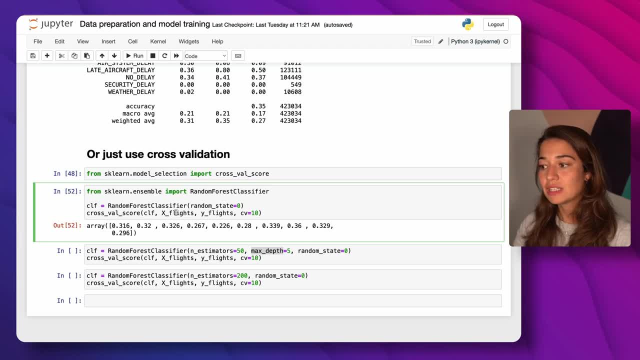 just initiated and the information and the data- x flights and y flights. What it's going to do is it's going to divide in itself this data into 10 different sub-datas and from then it's going to create 10 different. it's going to train using these values that you passed it, the hyper. 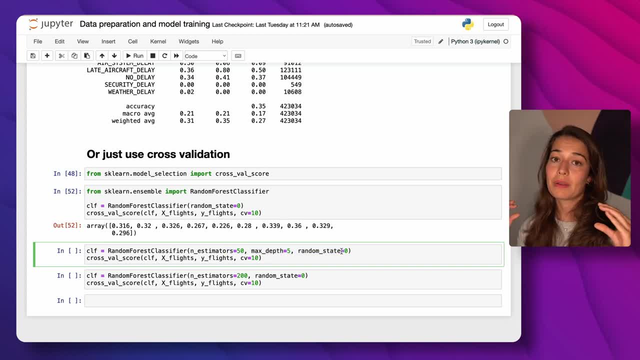 parameter settings, that you passed it 10 different machine learning models And these models will be reported here how well they perform. The reason that you want to do this is because you want to make sure that your model's results and performance is reproducible, and it is kind of 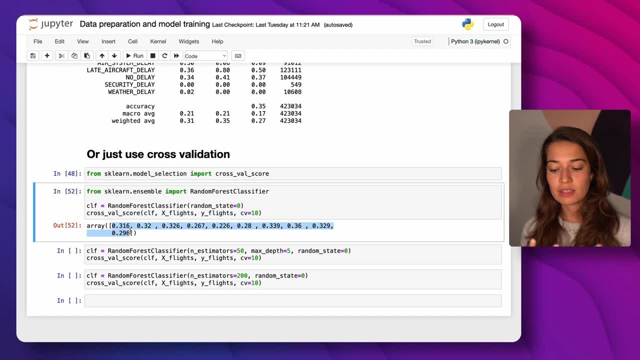 robust to changes in the data. So you want to see that your model actually understands the patterns in the data, instead of just fitting really well to one subset of data which is a subset of the real world that you're passing it So once you, if you want to make sure of that, you can use a 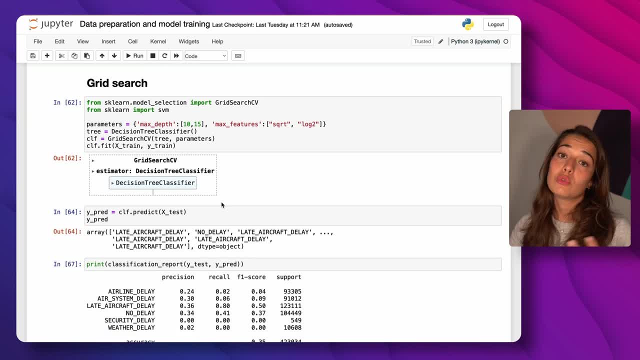 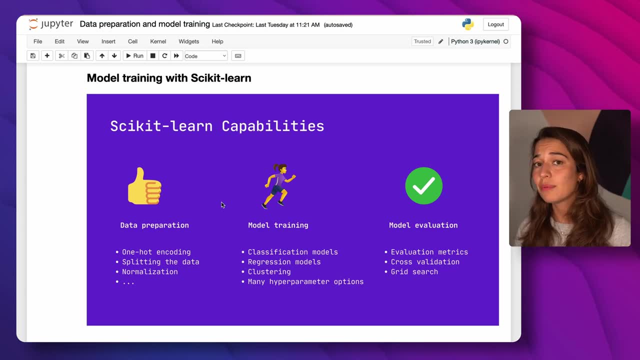 cross-validation score. but, as I said, if you're using grid search, it will already be included And these are generally the main steps of getting started with scikit-learn. As I said, it's a very big library. there are many things you can do with it.